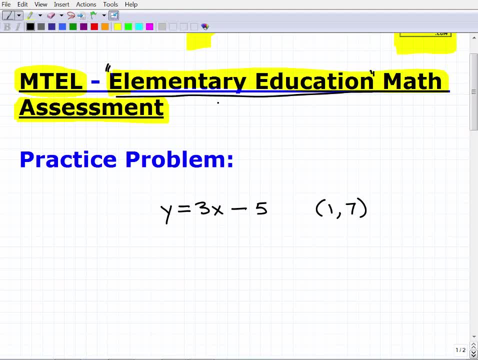 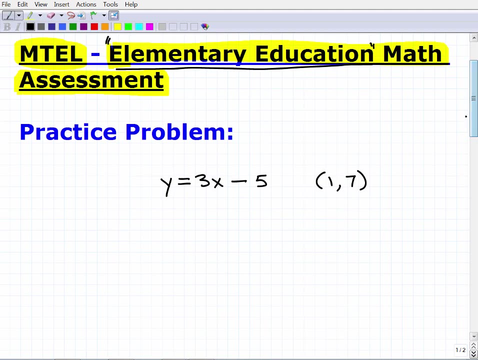 you're going to be facing. So, again, I would kind of characterize it as high school level algebra, geometry and some other kind of stuff. So you're going to have to really put some serious effort into brushing up your math skills to be confident on on this particular assessment. But with that being said, what I have here is a problem you should be able to handle for sure if you expect to do well on the MTL elementary education math assessment. So I'm going to give you a chance to solve it And then, of course, I'm going to go through it. So again, 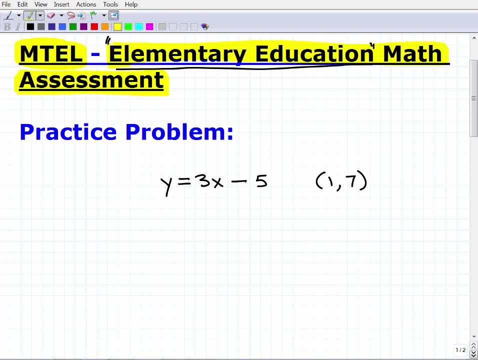 this is just kind of a quick spot check on one particular skill pop quiz, but let's have fun with it, Okay. so let me explain the problem to you And then let's see if you can do it. All right. So here I have an equation of a line. Okay, I want to know if this point is on that line. So I have a point. I'm going to explain this more here in a second, But I don't want to give you too many clues. So I have a point And I have an equation of a line. So my question is: is this point? 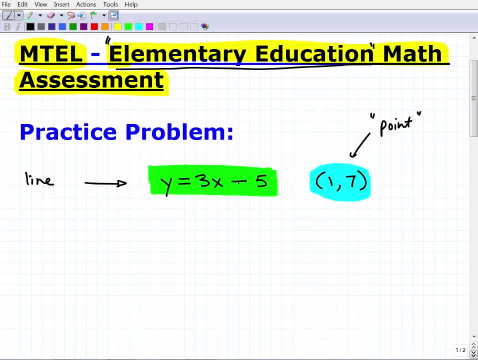 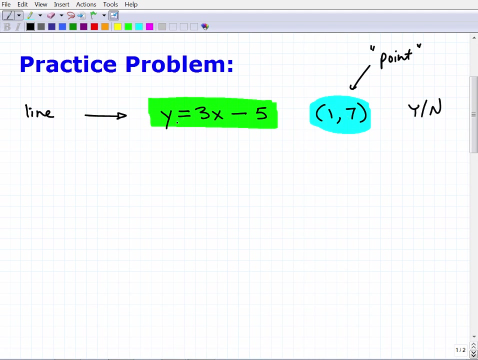 on this line, Okay, so kind of leave that there for a second. So hopefully a lot of you are going. okay, I understand the nature of the question And if you know how to solve it, I would encourage you to pause the video and solve it. Of course, I'm going to go through it And let's go through it now, Okay, so of course, the answer here is either going to be yes or no, correct? Well, it's either this point's either on this line or it's not. But let's, let's look at this problem visually And then we'll. 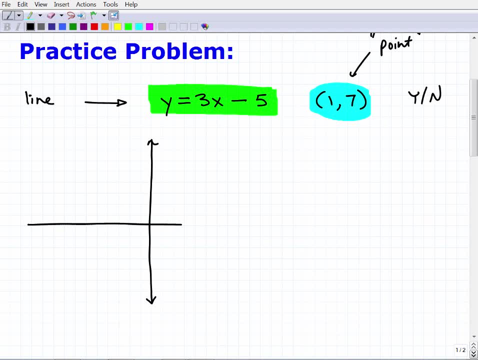 look at it algebraically. Okay, let me just kind of sketch this out And clarify. we know what we're talking about here. So I said this is a line. but really what we're talking about this is what we call a linear equation. So it's an equation, if you, if you just kind of listen to a linear equation. linear equation means equation of a line. So lines typically we like to write in y equals mx plus b format. Now, if what I'm 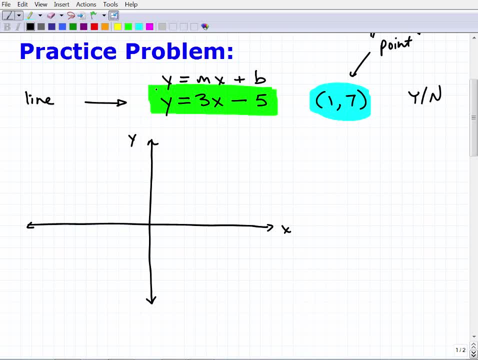 talking about here. if you're kind of lost, you know then that's a strong flag, red flag, that you got a lot to learn, you know to prep for this exam. If you kind of vaguely kind of understand what I'm saying, you're like, Oh, I kind of remember that from my high school- math or college. you know one of your classes and that's good as well. But the main idea here is, if you kind of somewhat know what I'm talking about, that's not good enough either. you're really gonna have to know this very, very well, along with several 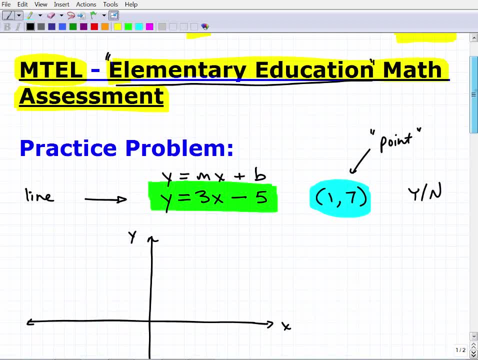 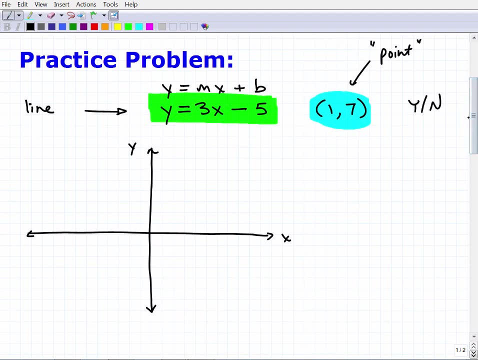 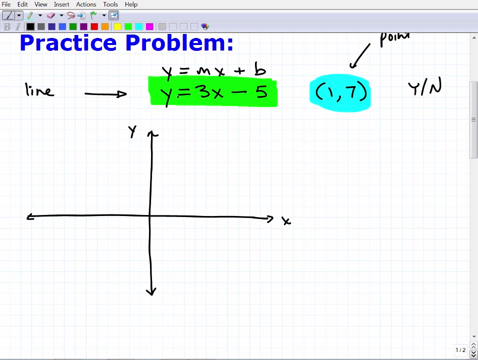 other math topics. So again, you know we're talking about a professional certification exam here. you know you have to really study for these assessments. I'll talk more about that later. So yes, there is a decent amount of math, for sure. that's on these assessments. But let's continue back with the problem. So what I'm going to do is I'm going to graph this line. Now we can kind of turn this into the second question here in this problem. If you think you can graph this line, I would encourage you to just 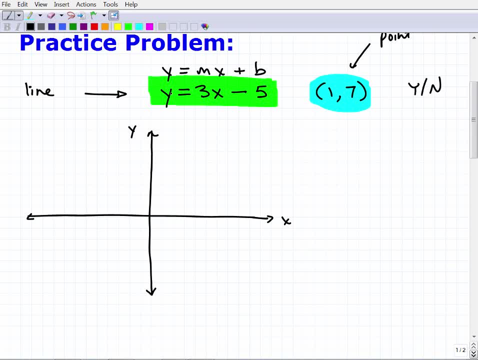 quickly sketch it out and graph it on. you know, just draw a little xy plane, like I did, and then graph it out, And then I'm going to plot this point one seven. So I'm going to go and do this now. So I'm going to start at negative 512345.. I don't want to turn this lesson into complete, you know. you know full lessons on graphing lines and all this other stuff. So I'm going to be skipping some things here. So I'm just graphing this line. So I'm going to start here at negative five, which is the y intercept. 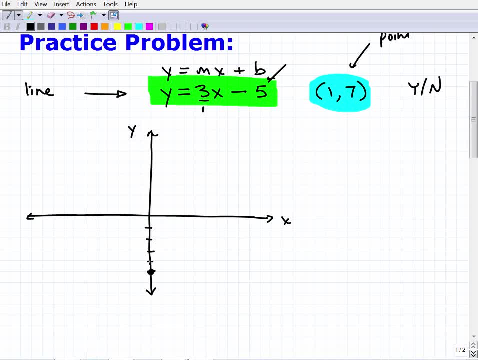 And then I'm going to go up three and over one. I'm using the slope here. So one, two, three over one. So that's the second point. So these two points are on this line And now I'm just going to hopefully do a pretty good little sketch through those two points. Okay, so this is a rough sketch of the line of this linear equation: y equals three, x minus five. Okay, so this is the graphical representation of this linear equation. So the question I'm going to ask is: how do I get this line? 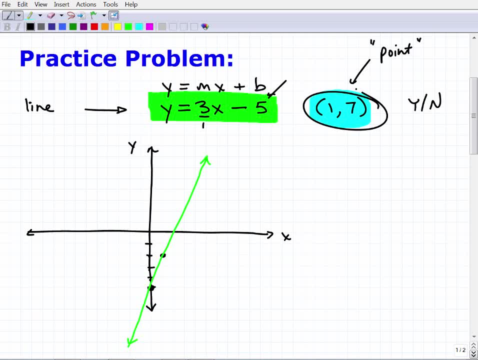 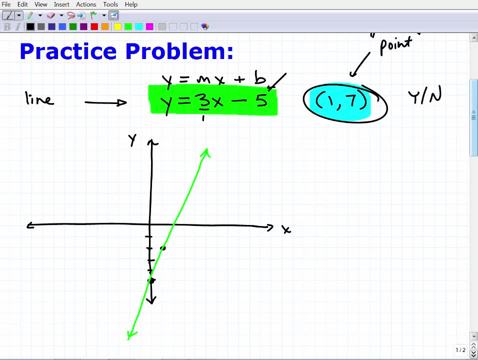 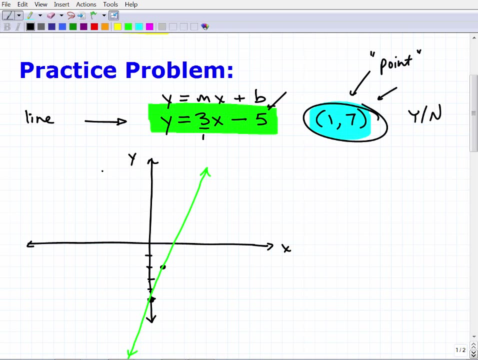 I had. the original question is the point 1, 7 on this line. now we can just take a look at this point and graph it. now, these points in algebra, there they go by different names. okay, so point or coordinate- okay, which would be another point on the coordinate plane, but I like the term ordered pair. okay, so an ordered. 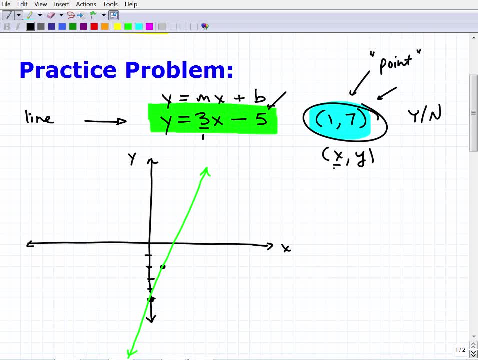 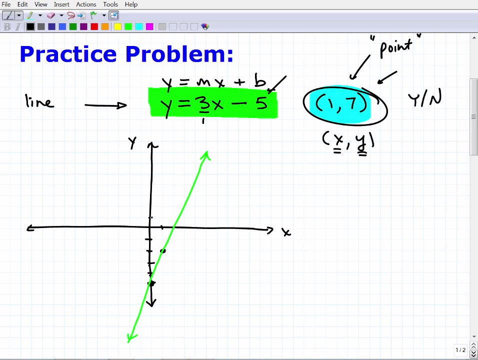 pair is a pair of numbers, the first being the first in the two, the pair. here there's a specific order. the first is the x-coordinate and the second is the y. so here this one. I would go over one on the x-axis and then seven on the y, so 1. 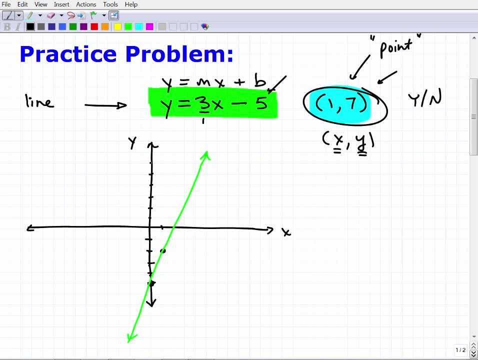 2, 1, 2, 3, 4, 5, 6, 7. all right, so here is roughly the ordered pair or coordinate or point: one seven. so we have one seven. so we have one seven. we have this sketch of this line. so, assuming I you know working with the 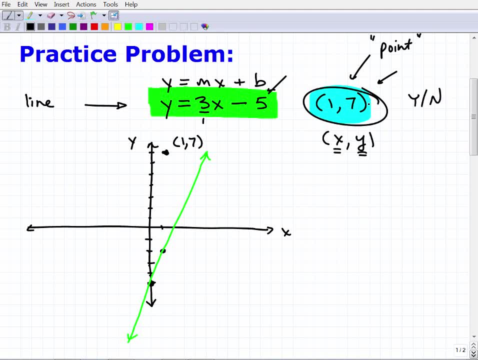 pretty accurate. you know graph paper or whatnot. we can kind of add, you know, answer the question visually right. so is the point 1, 7 on the on the line y equals 3x minus 5. well, clearly not right. this point is not on this line, so the 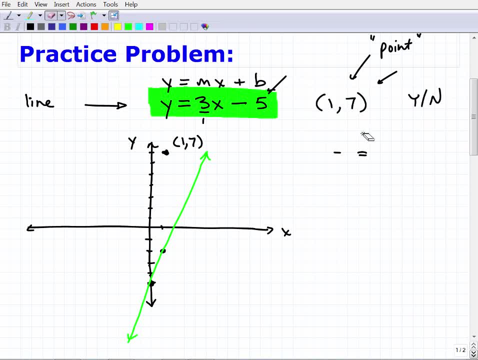 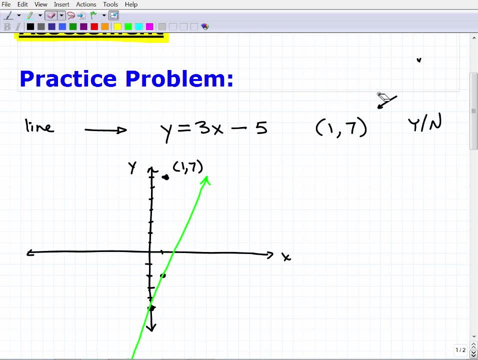 answer is no. but now let's answer this question algebraically, okay, so let me kind of erase all this. so, if you're with me, so far new and that's excellent, okay. so what am I going to do? well, again, remember, I said this is X and this is Y. okay, we're talking about an. 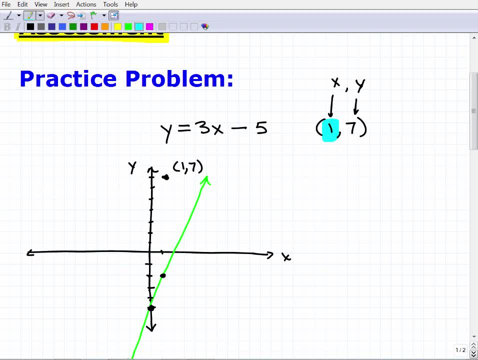 ordered pair. well, if I plug in this X here, where this X is at in this equation, and this Y value right here, okay, so this is one coordinate, one ordered pair. if I plug it into this particular equation, what I should get is that the left hand valve- uh, mark values of the igual Memąt is in the left hand diagonal. aba u Izic means power. 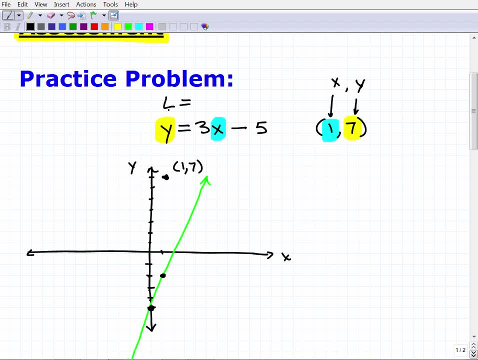 side of the left-hand side of this equation should equal to the right-hand side. It should balance like any equation, right? It's an equal sign here, So let's plug this in. So let me write this down here: y equals 3x minus 1.. So I'm going to replace the y with the 7,. okay, So that's 7.. 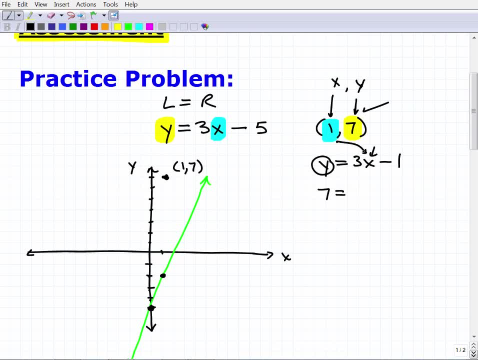 Then I'm going to replace this x here with this 1.. So that's going to be 3 times 1 minus- oops, this should be 5.. I apologize about that. Always double-checking your work, So this should. 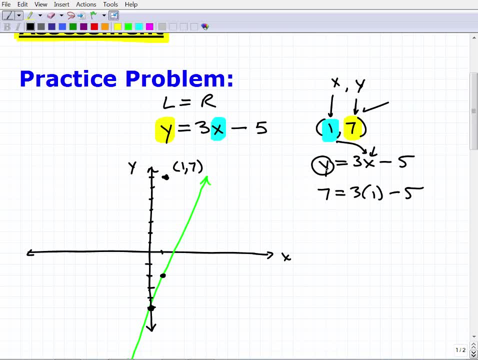 be, that's minus 5,, right? So here we go. So I replace the y with the 7, and I replace the x with the 1, and I just wrote the original equation, Then what I'm looking to see here. 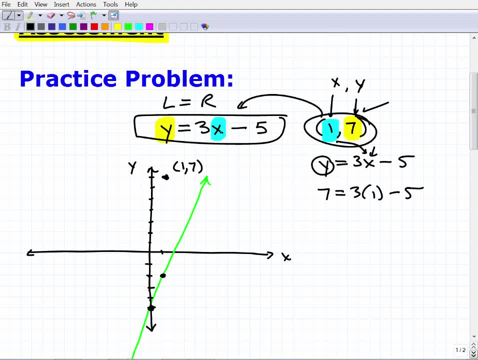 does this point when I plug it in for the respective x- y values, is it going to balance? Okay, so what do I get here? I get: 7 equals 3 times 1 is 3x, So 3 minus 5, is that true? So 7 equals negative 2? Well, no, okay, That's false. This is a false. 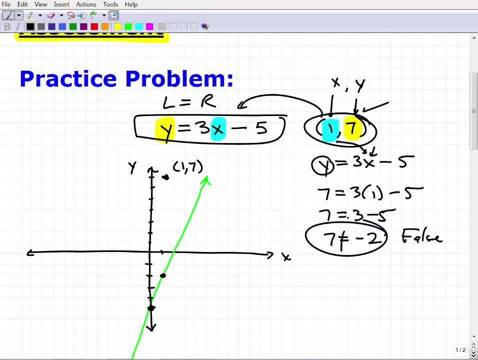 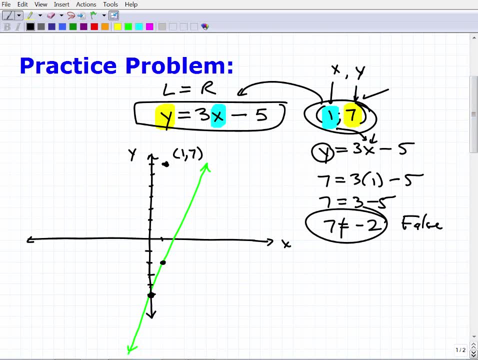 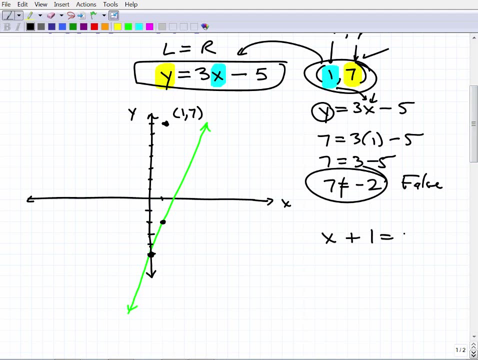 statement. So because this is false, all right. when I plugged in these values here because it didn't balance the equation, then this does not lie on that line. It would be very much like this If I give you an equation like: x plus 1 equals 4.. 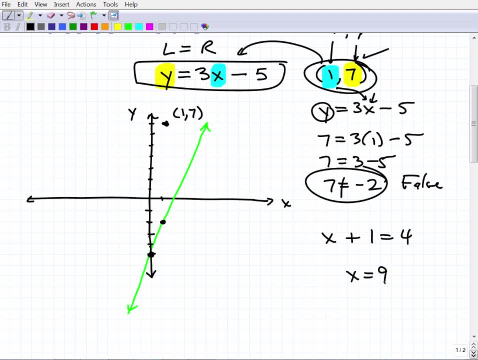 And I'm going to say: is x equals 9? the solution to this equation? So: is x equals 9? the solution to this equation? Well, you would just replace this x with a 9, so you would have 9 plus 1.. 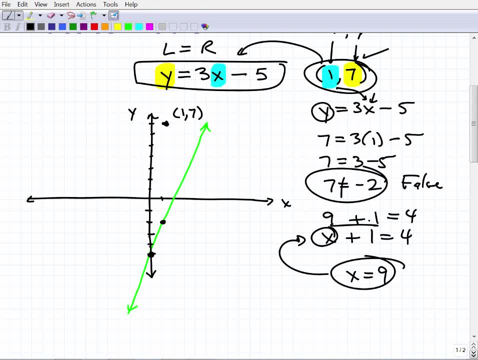 And we have to ask ourselves: does 9 plus 1, does the left-hand side in fact equal the right-hand side? No 9 plus 1 is 10.. 10 does not equal 4, so x equals 9 is not the solution to this equation, And this is the same kind of 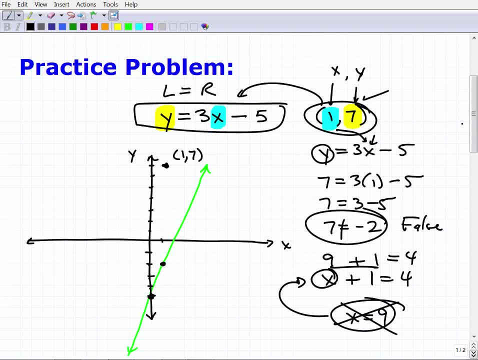 logic that we use to answer a question like this. So real basic algebra stuff, graphing lines, and there's much, much more that you're going to have to be proficient at. But you know, this was a kind of a quick little review. We kind of hit a few real important. 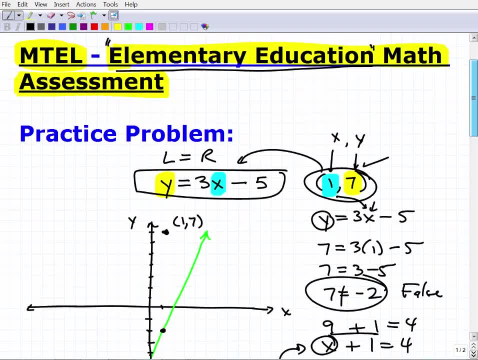 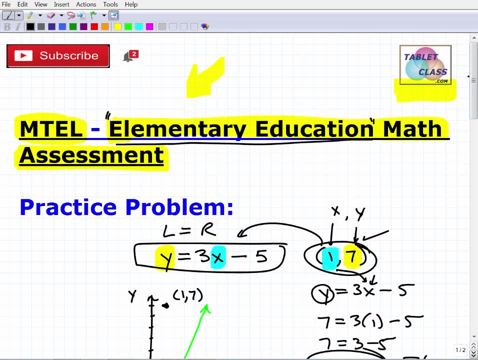 topics. Again, you know I can't turn this video into a complete, full lesson on a lot of these important topics. That's what I encourage you to. you know, get yourself into a good study program and give yourself enough time. If you don't have enough time, you can do it in a few minutes. So I'm going to give you a little bit of a quick review And I'm going to give you a little bit of a look at this. And I'm going to give you a little bit of a look at this And I'm going to give you a little bit of a look at this. 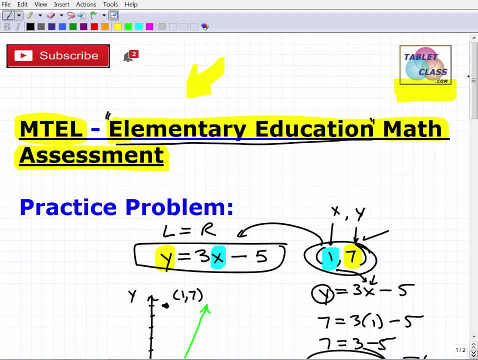 and give yourself enough time, if you have the time, to study, practice and just kind of brush off All the stuff that you're going to need for the MTL Elementary Education Math Assessment. you've studied somewhere in your past, okay, in high school or in college, the majority of it, for sure. 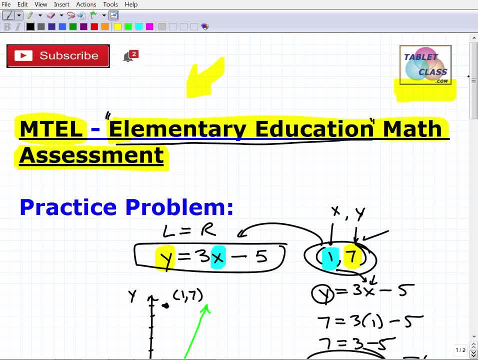 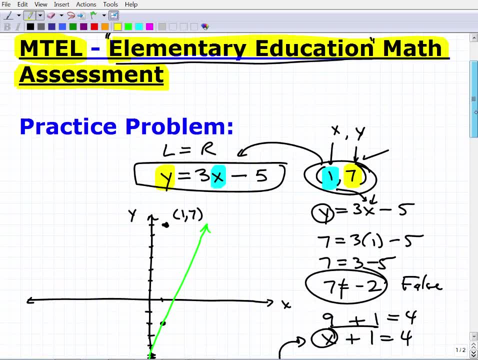 You just probably don't remember a lot of it, and that's completely normal. But you're going to have to certainly brush up on your math to get through this assessment with flying colors, And that was the goal of this video. So I'm just going to wrap it up. 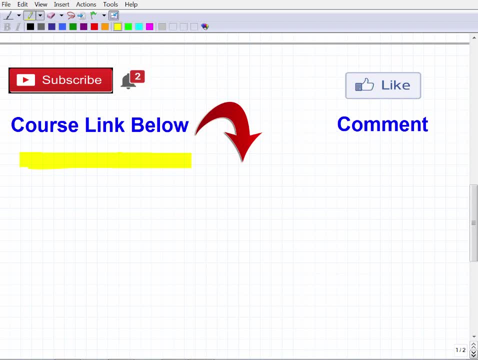 So a couple of thoughts here. So again, if you want to check out my test prep course on this, the MTL Elementary Education Math Assessment, I'm going to leave the link to that in the description of this video. I've been on YouTube for like 12 years, plus at the time of this video. 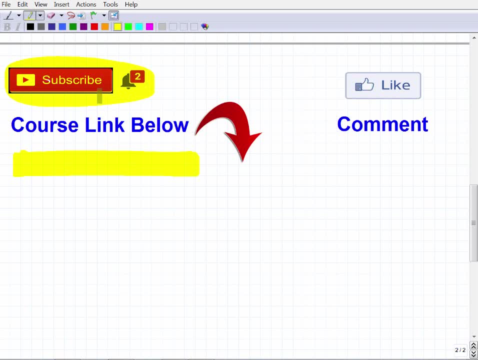 I literally have hundreds and hundreds of videos I can help you prepare And I think I'm pretty proud of the fact that I think I have like 13 million total views And a lot of subscribers- well over 100,000, like 125,000, 126,000. 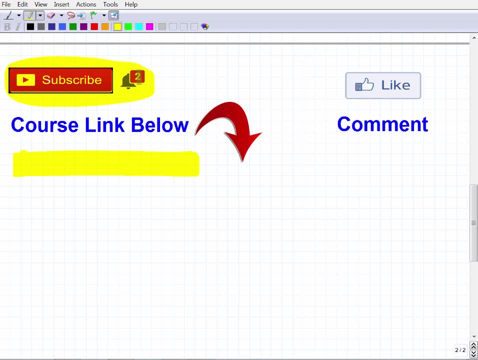 I only say that because you know it just goes, you know, to for me my passion for teaching math. okay, And when I started teaching and sharing videos and just doing tutorials and stuff, I just put so much information out there. 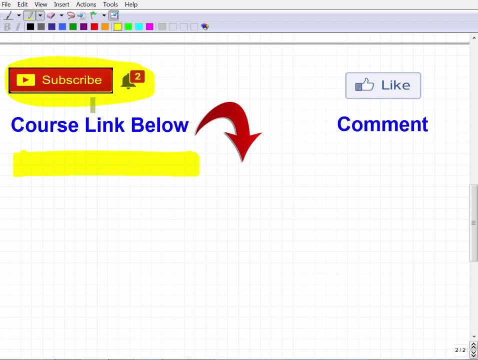 I basically put things out there to help people, And I've been doing it for a long, long time, So I've really built up a significant amount of math. I've done a lot of tutorials that can definitely benefit anyone, So check that out if that's something you want to check out. 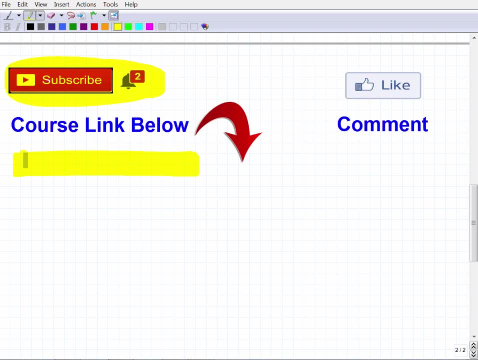 You can definitely subscribe or just check out my playlist, Or you can take my. you know, check out my full comprehensive course. That's my best work. Hey, if you like this video, definitely appreciate a thumbs up And leave me some feedback. 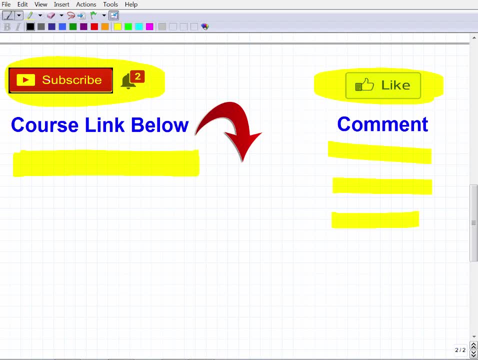 You know, is this your first time taking this exam, You'd be surprised that it's not uncommon at all for teachers that have to take certification assessments more than once. okay, So if this is your first time taking this exam, you're going to be surprised. 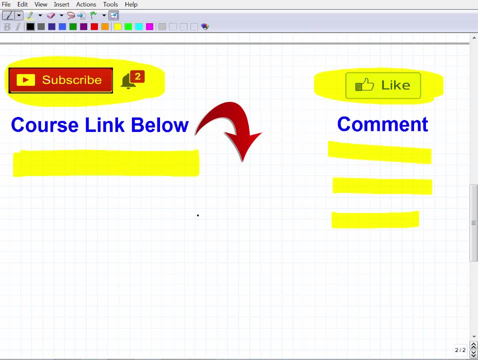 If this is your second time you know, or even your third time, don't let that stop you, okay, Because there's a lot of people out there that have to, you know, retake exams. okay, I know, for my particular exam, I actually took the Praxis exam for high school of math.